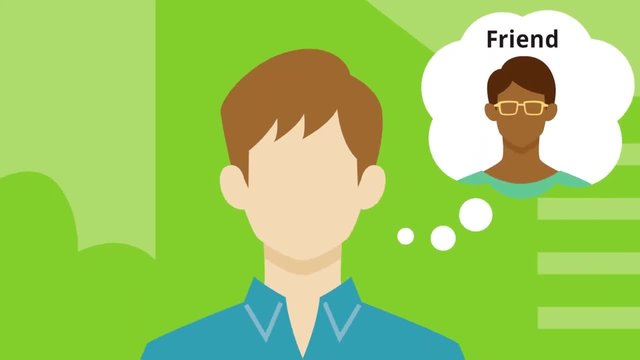 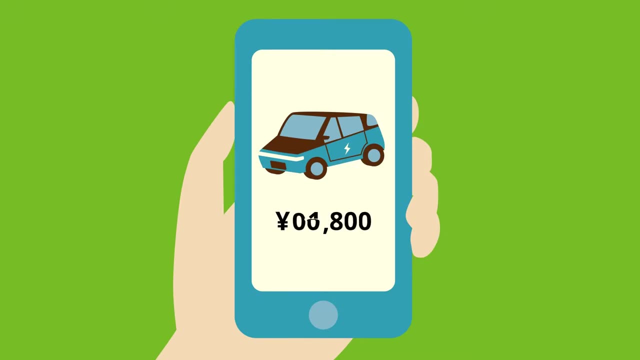 Today he plans to go for a drive with a friend. To do so, he first needs to hire a car. Previously, a flat rate was offered to all customers, Whereas in the future you can get a discount by proving that you are a low accident risk. 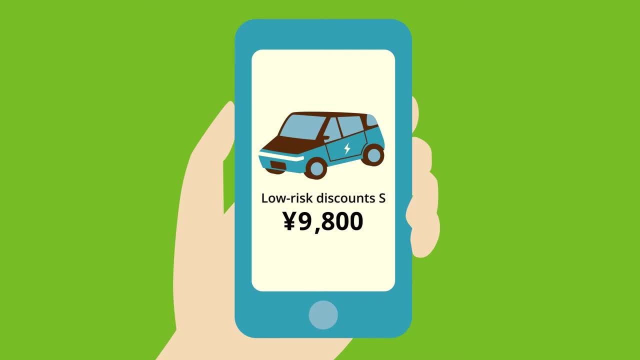 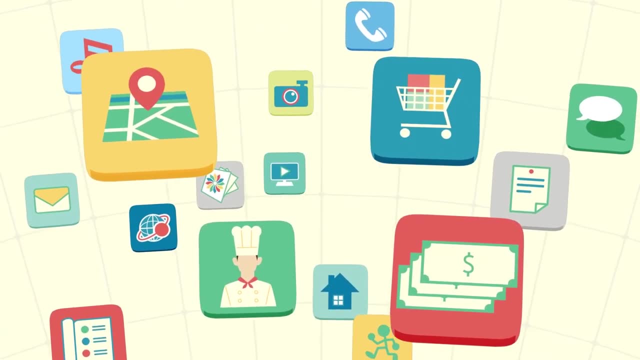 There is enough data in the user's device that can help determine the level of accident risk. However, some data could be misused if leaked, So one must be careful. It is important to be careful not to reveal all data to the car rental company. 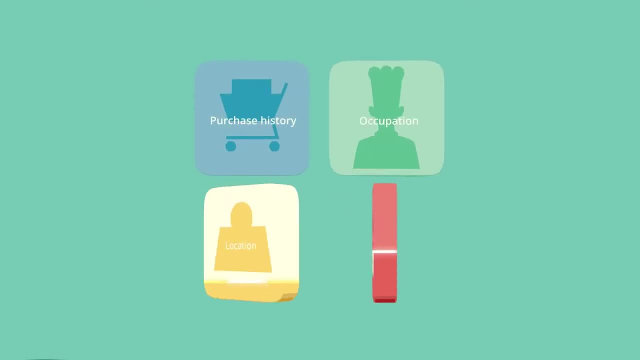 Privacy-enhancing technologies can be used to process the data into the minimum amount of information required for calculating the accident risk on the user's device before being submitted. The car rental company can trust the processed information, as it can receive a certificate of this process. 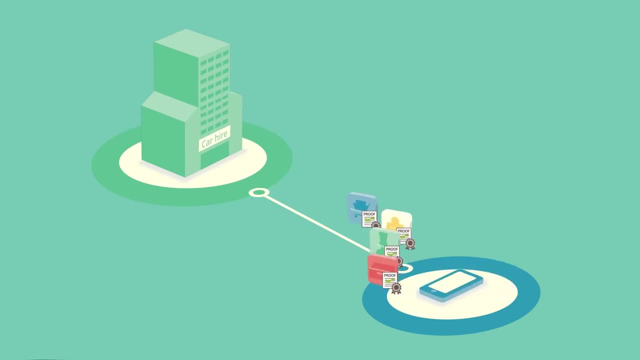 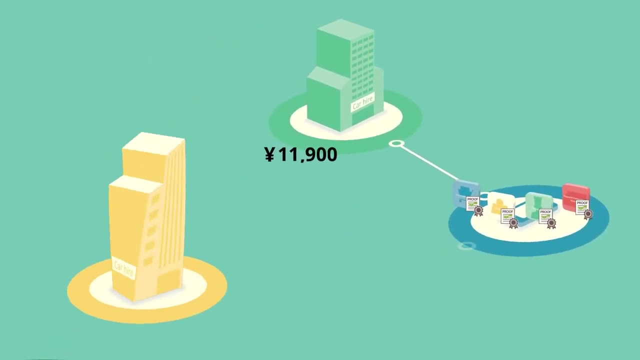 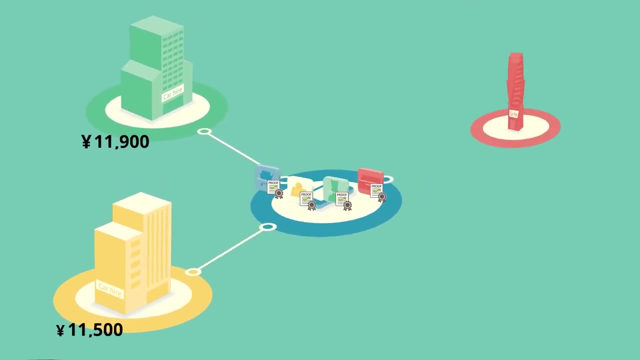 The car rental company is then able to offer a price appropriate to the submitted accident risk. Computer performance has improved dramatically over the years And multiple companies can offer personalized rates within seconds. The competitiveness of a company depends on how well it can offer the best rates. 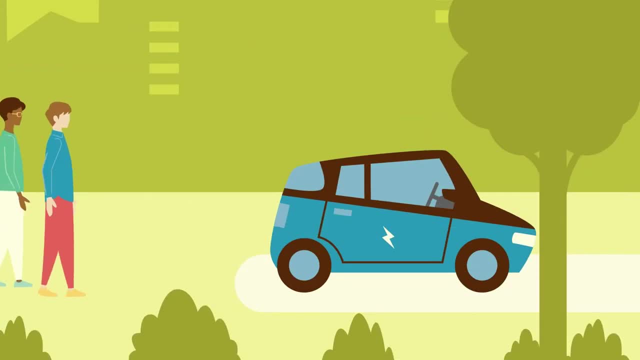 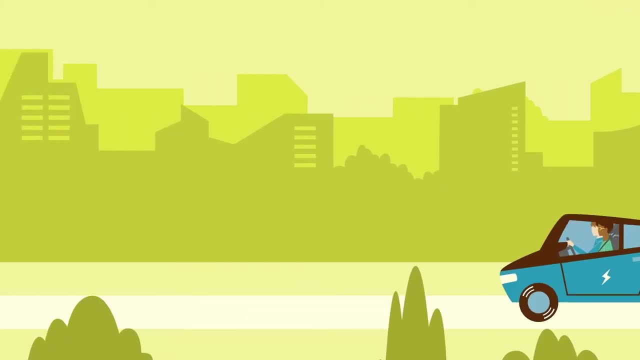 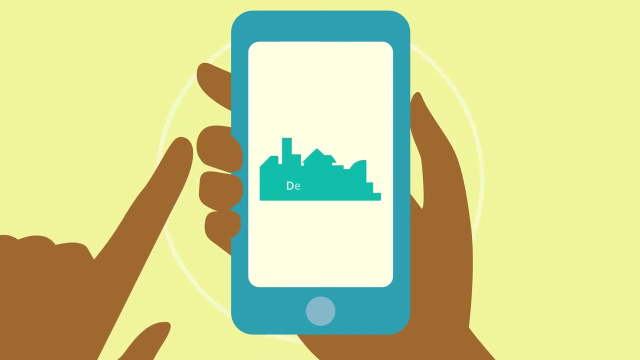 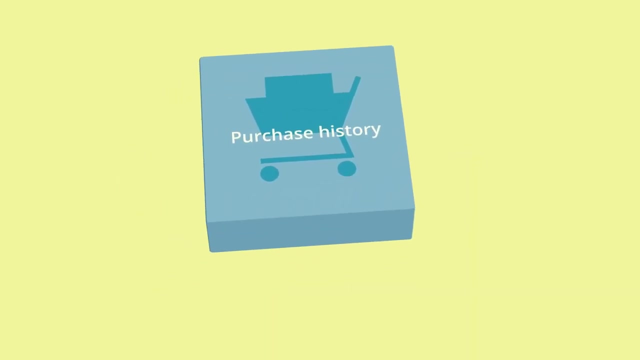 In this case, they have decided on this company. They may have a little extra time on their hands. In such an instance, they ask the application for a detour destination that they might enjoy. Smartphones now store lots of data processed by privacy-enhancing technologies. 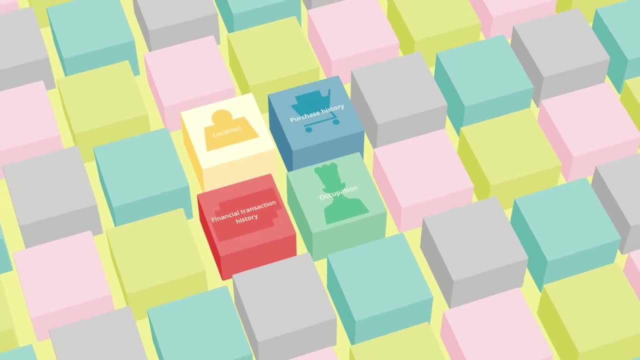 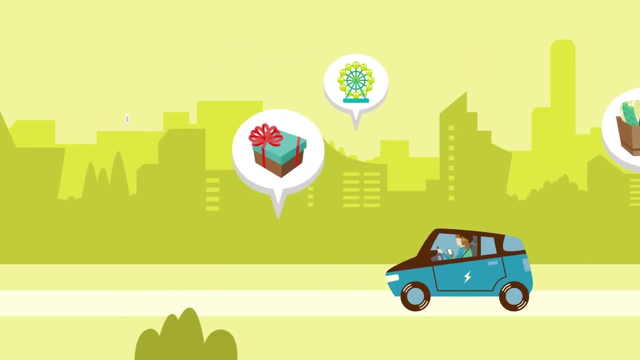 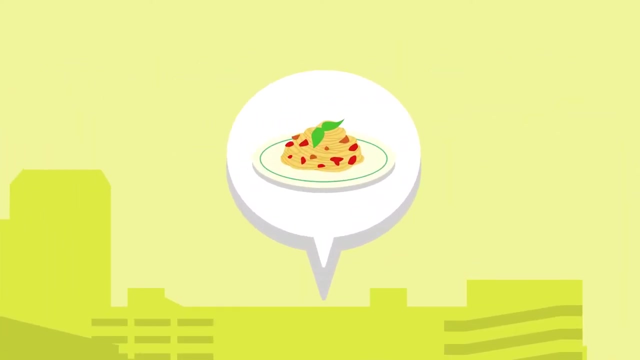 Users only allow this data to be used for ad recommendations, So advertising companies are competing with each other to show users the best adverts from this data. They were attracted by this restaurant's popular menu. having arrived at a shopping mall, The restaurant they want to visit is here. 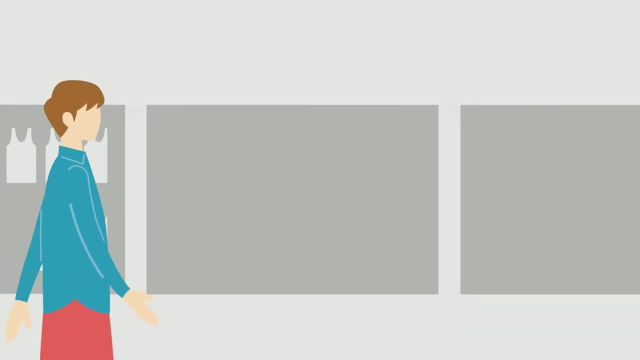 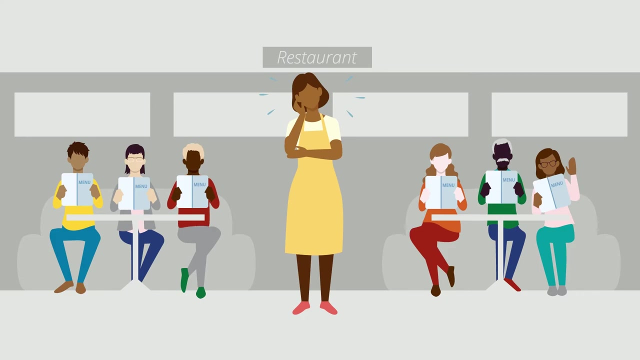 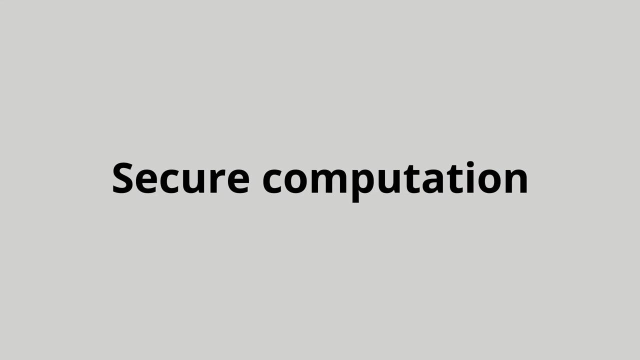 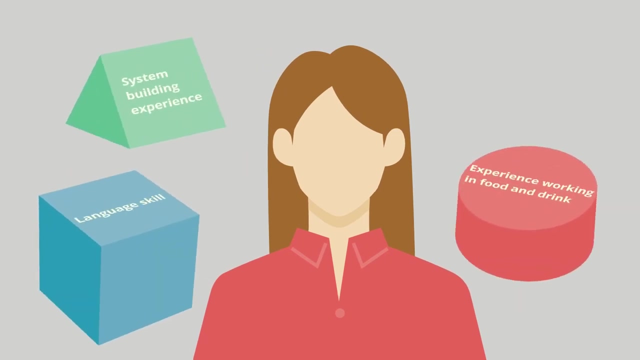 However, this restaurant seems to be in trouble due to a sudden staff shortage. We can all be useful to someone. You could register the skills you possess. You may be offered a job at short notice in your neighborhood. The skills information registered by the user is kept confidential by privacy-enhancing. 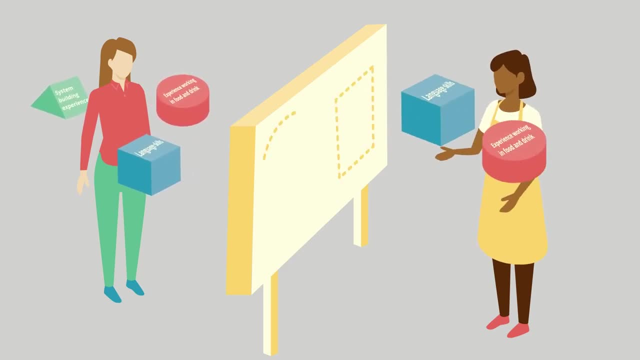 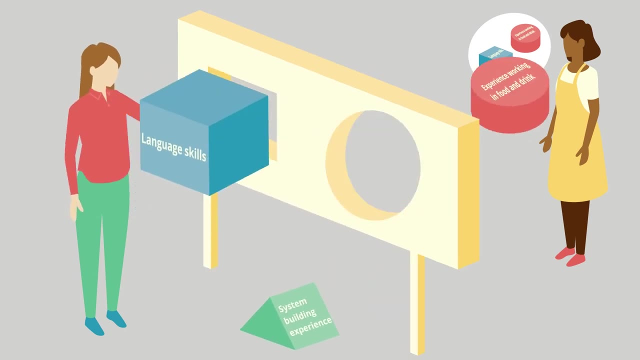 technologies and is only passed to the other side when there is a match to a job offer. so you can register without a care. We can all be useful to someone. You could register the skills you possess. You can also choose them as your personal interests and we can trust you. 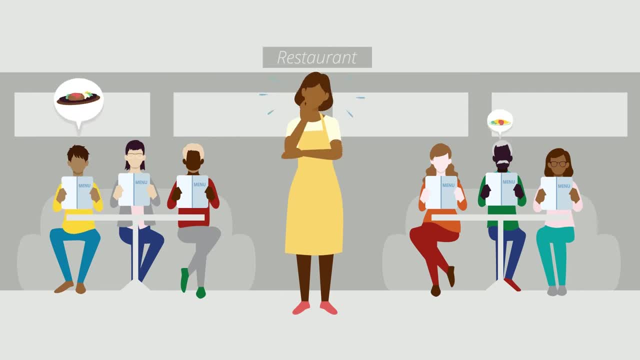 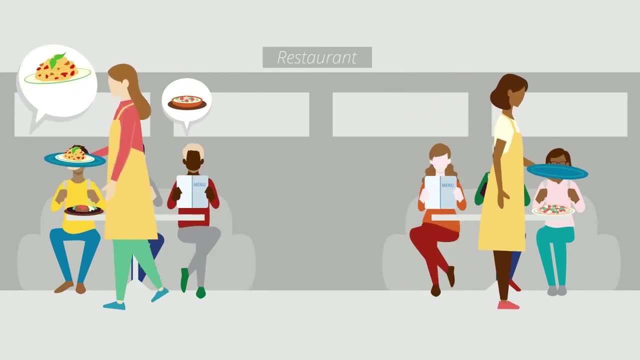 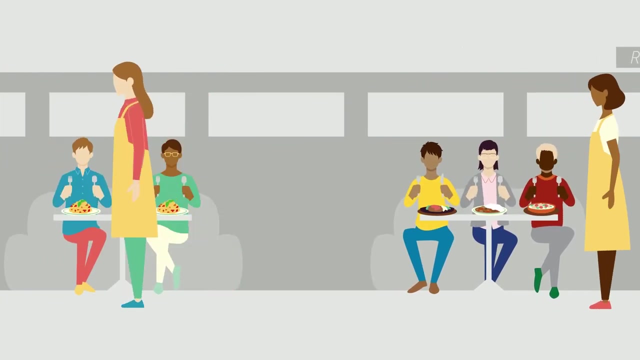 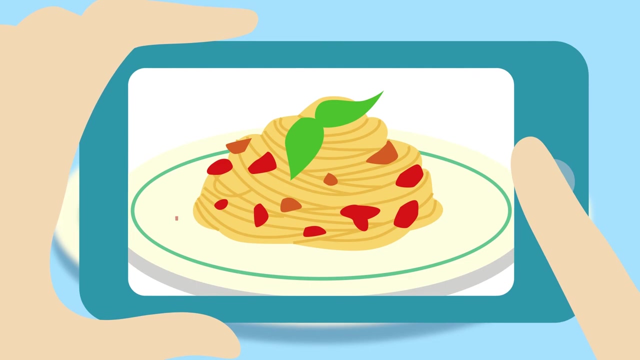 So our time is over. Thank you, Bye, bye. Advertiseer. you know it's hard like this. Watch the next part on Music Bank. Everything so far from this session of Number 일� Kesummary is my way of getting to the point on your favorite specific topics. 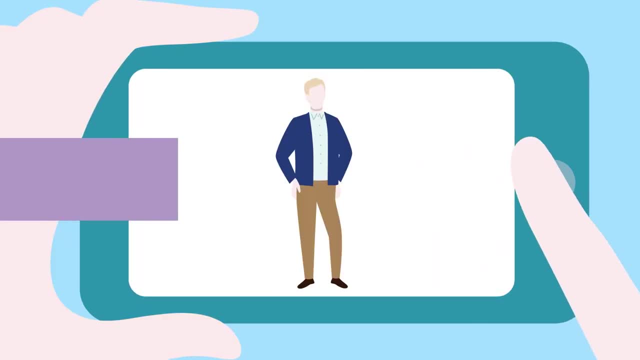 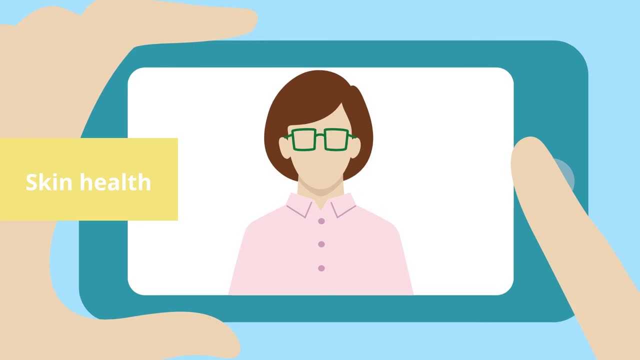 Thank you for watching And you're all welcome to check out our next headlines for Director: Commercial Video with chronic illnesses. Photographs of non-food items can also provide information on various health conditions. Companies want their employees to stay healthy, so they subsidize products. 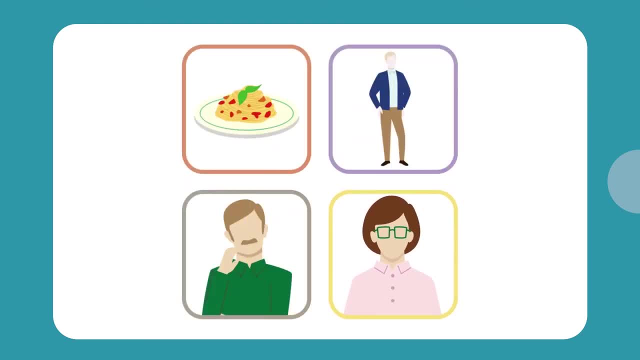 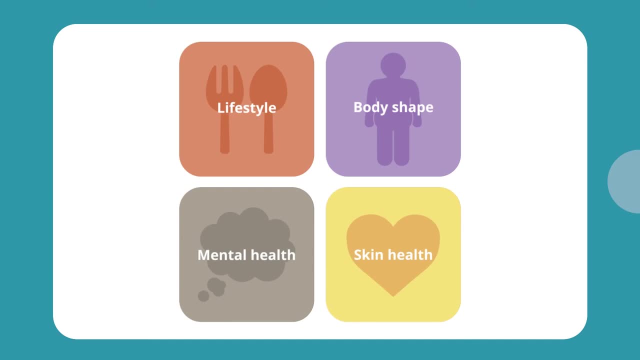 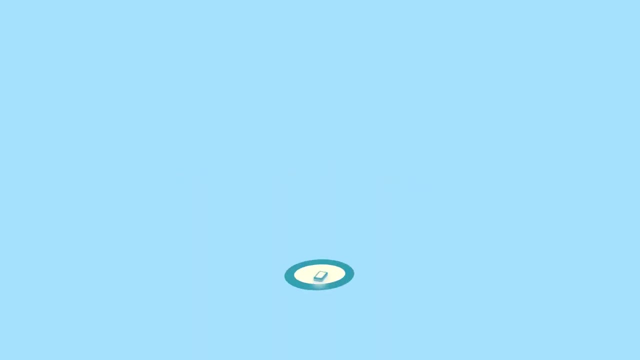 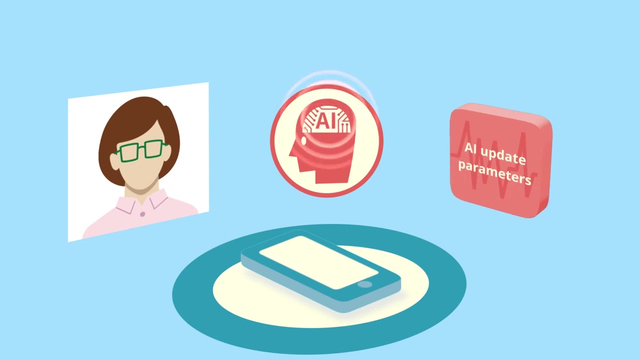 of partner companies for those who have undergone a health risk check by photos, according to the results, in an effort to improve the well-being of their employees. The leaking of photos cannot happen because the analysis is carried out in the user's terminal by cloned AI sent from the company to the user's terminal. 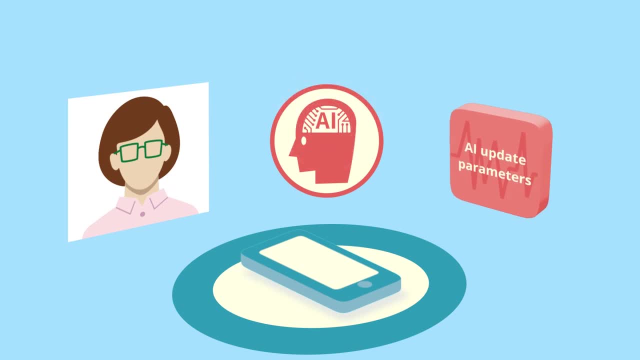 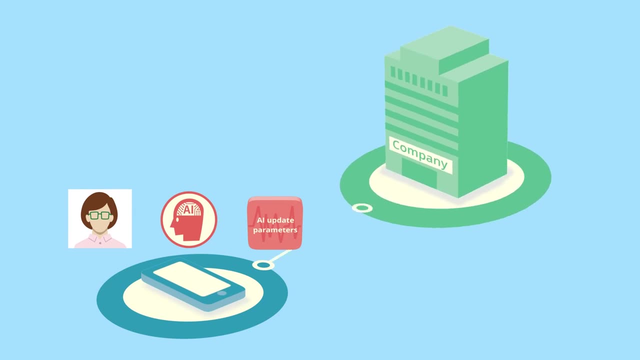 The cloned AI in the user's smartphone performs better than in the case of a photo. The cloned AI in the user's smartphone performs better than in the case of a photo, ichtet to machine learning to do with risk analysis and feeds back parameters for updating the company's original AI. It is not possible to revert these parameters. 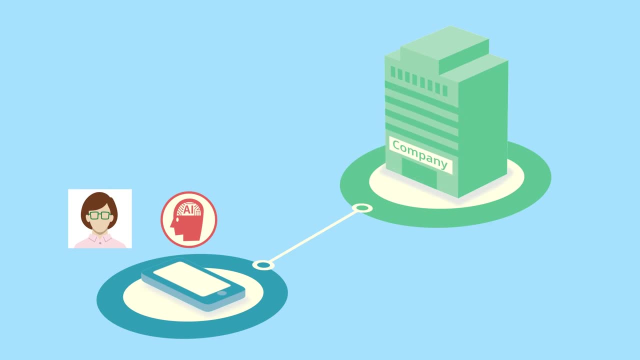 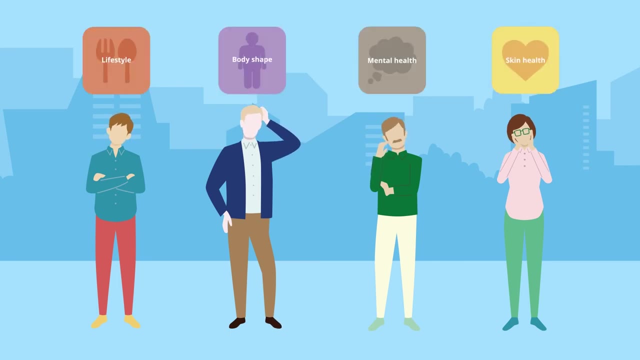 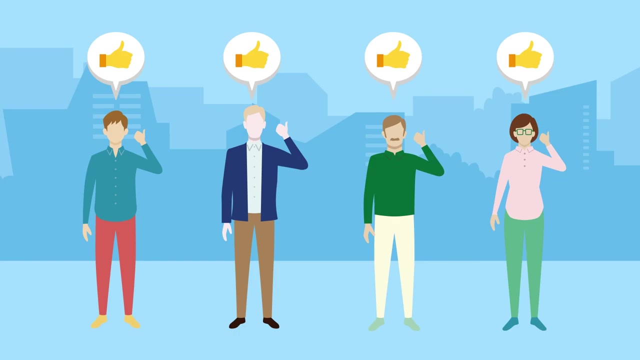 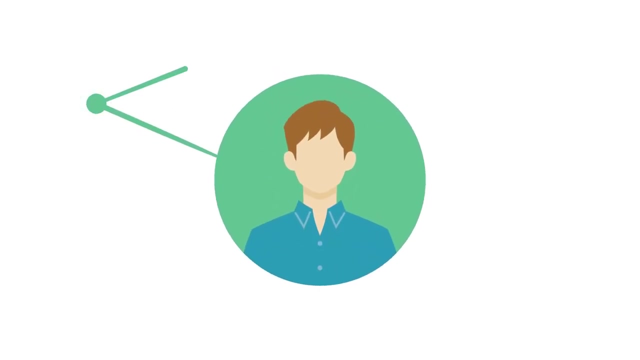 back to photo data. A careful explanation of this method has made it possible to expand users to those who are not comfortable using private data, such as photographs for analysis, PDF, torture. This is the scenario we envision Once leaked privacy information is more easily disseminated and harder to undo than before.